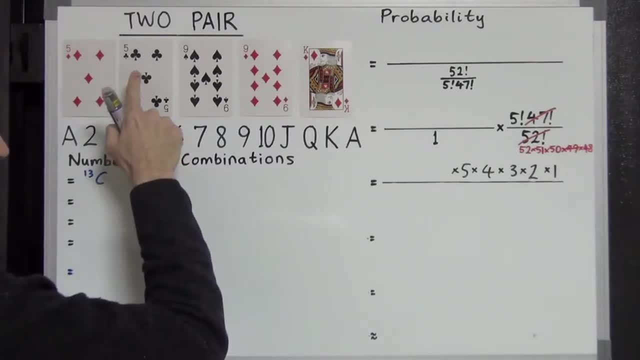 13 c, and we have actually have to choose two ranks for the first pair and the second pair: 13 c- 2. and then for our first pair, we have four cards to choose from and we choose 2, 4 c, 2 and the same for our second pair, times 4 c- 2 and left over. 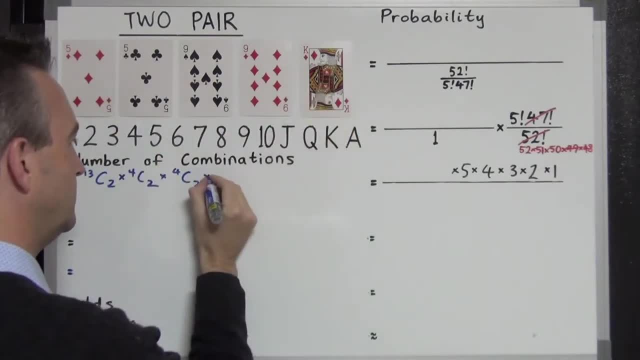 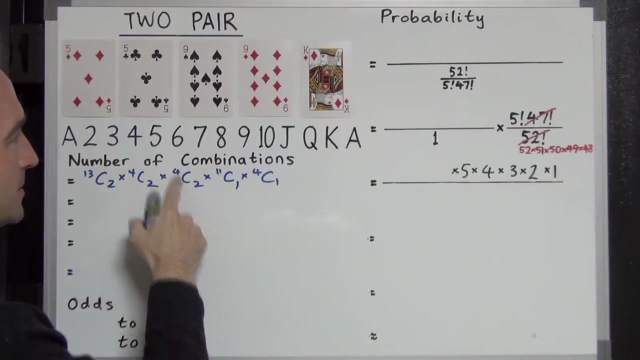 our two ranks are already gone, which leaves us 11 ranks to choose from. and if we're doing kings here, we have four kings to choose from. we need to choose one Question: can we not do 13 c 1, 4 c 2 and then 12 c 1 times 4 c 2 for our two pairs? Yes, you can, but then you're gonna. 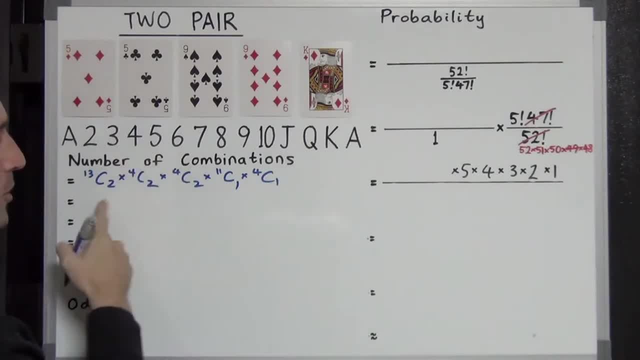 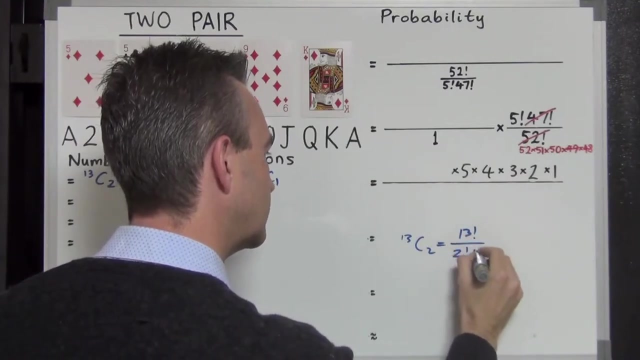 actually have to divide by factorial 2 in the end to undo that permutation. If you want to see a better explanation of that, have a look at our one pair presentation Evaluating this: 13 c 2. oh, what's that? 13 c 2, factorial 13, factorial 2, factorial 11.. 13 and 11 cancel 13 times. 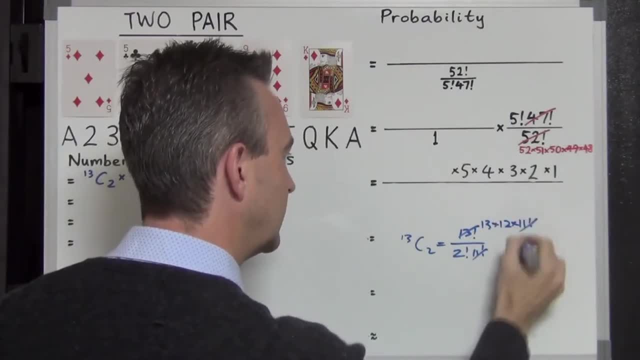 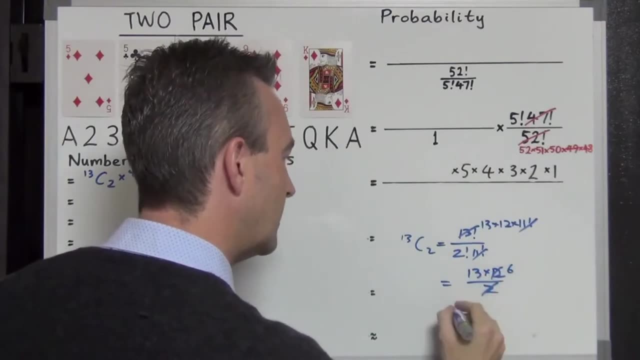 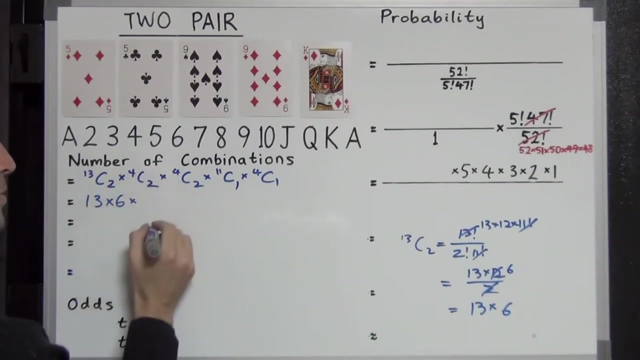 12 times 11.. factorial: it cancels there now, leaving 13 times 12 over 2. 2's cancel, giving 6. 13 times 6.. I might just leave it like that and write it straight in here: 13 times 6.. 4 c, 2 is. 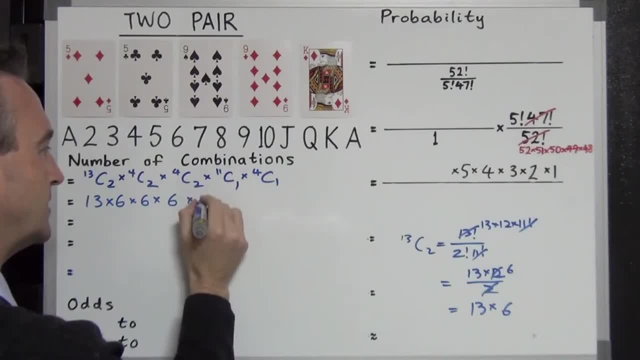 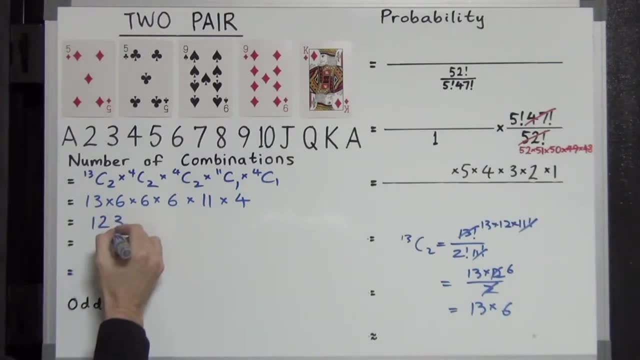 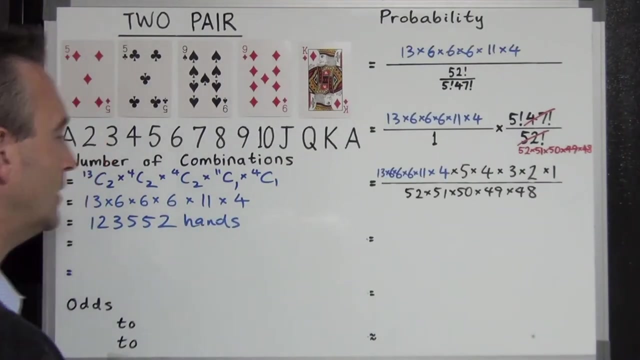 6.. 4 c- 2 again is 6, and then 11 c- 1 is 11.. 4 c- 1 is 4.. Evaluating that, that is 123 000.. 552 000.. To calculate the probability of getting two pair, we're going to take this expression here and write: 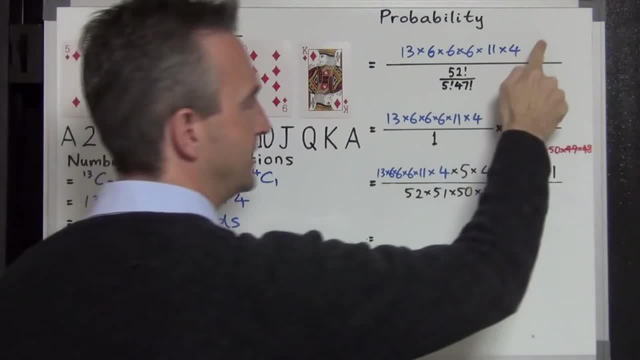 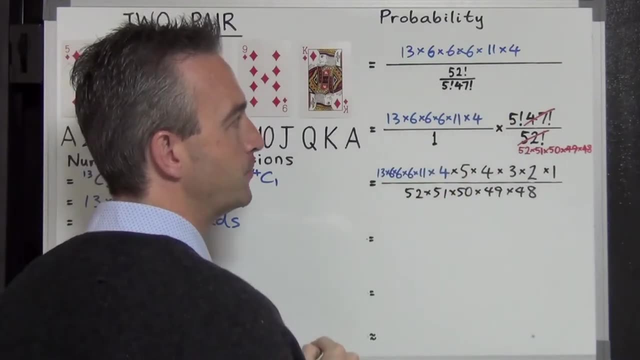 it up here, but i'm going to take this expression just for ease of cancelling later on. number of two pair hands divided by- and this expression here is 52 c 5- the number of possible poker hands dividing by this gets inverted and multiplied and 47 factorial cancels. 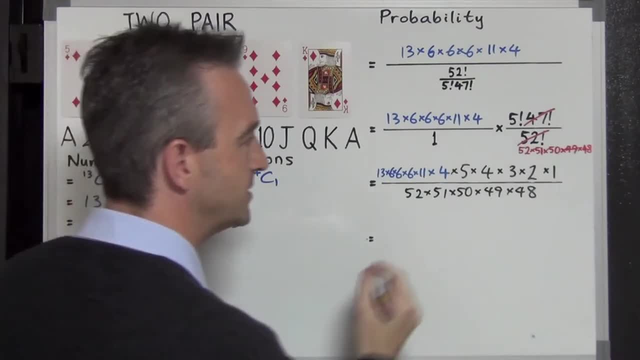 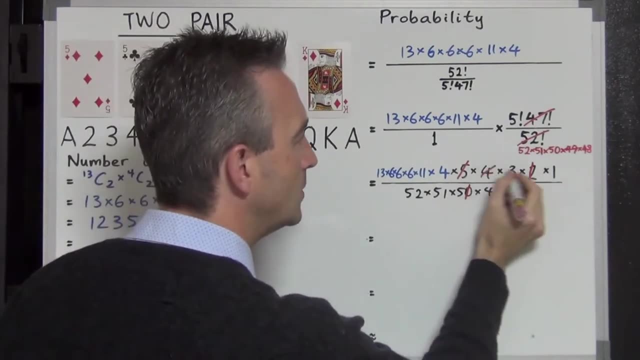 leaving us with this expression here, and let's see how this cancels out: 5 c 2.. 5 c 2. 2 will cancel with the 10 here, just leaving 5 instead of 50.. 4 times 3 is 12, times 4 is 48, that will cancel with 48 at the bottom. 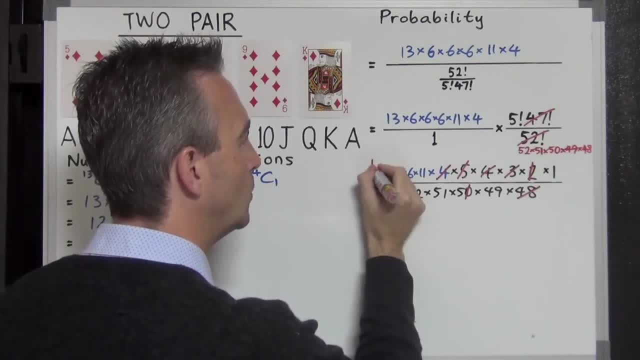 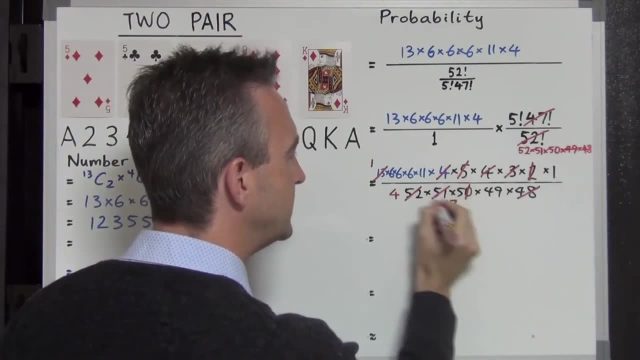 What else do we have? We have a 13 goes into 13 once, 13 goes into 52 four times. And we have a 51,. 3 goes into 51 17 times. 3 goes into 6 twice. 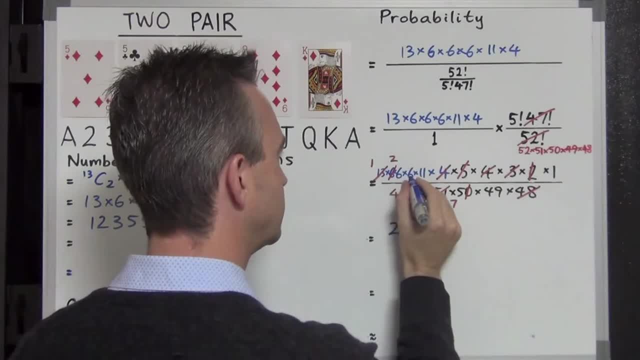 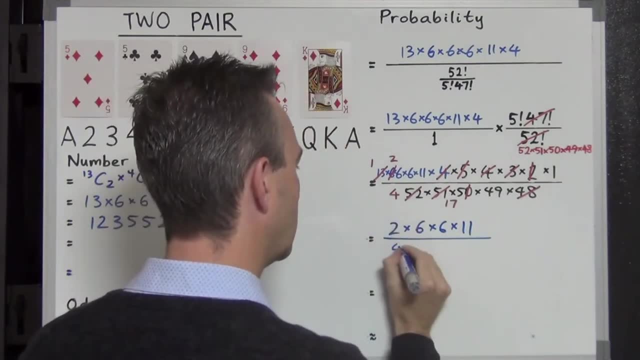 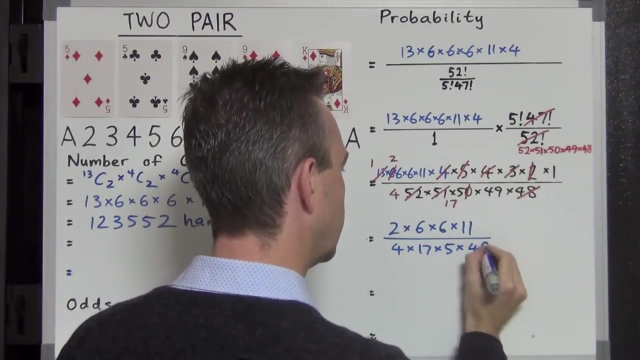 That is it, I believe it leaves us with 2 times 6 times 6 times 11.. That is all there is on top, and on the bottom we are left with 4 times 17 times 5 times 49.. Oh, that is not finished. we can go further than that. 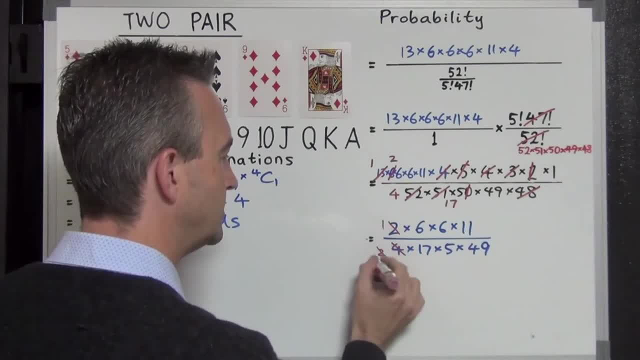 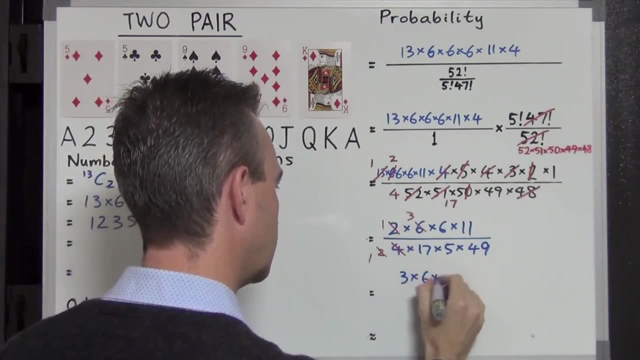 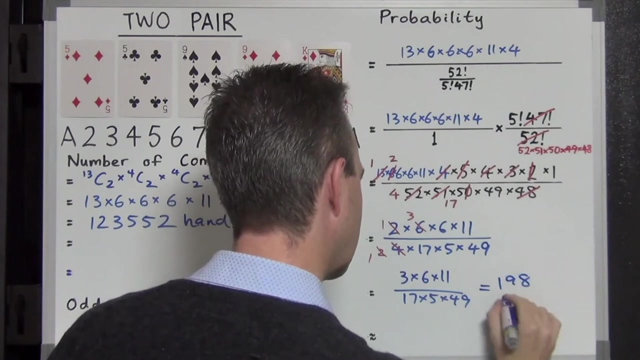 2 goes into 2, once 2 goes into 4. twice 2 goes into 2, once 2 goes into 6, three times, Leaving us with 3 times 6 times 11.. Over Over 17 times 5 times 49, which gives us a final probability of 198, over 4165, which 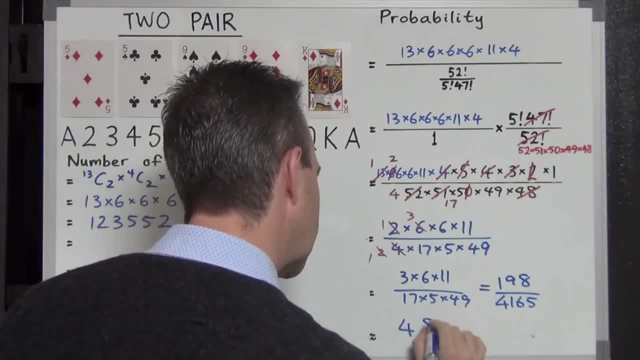 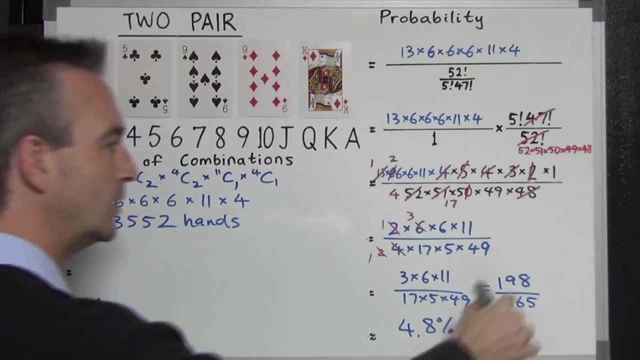 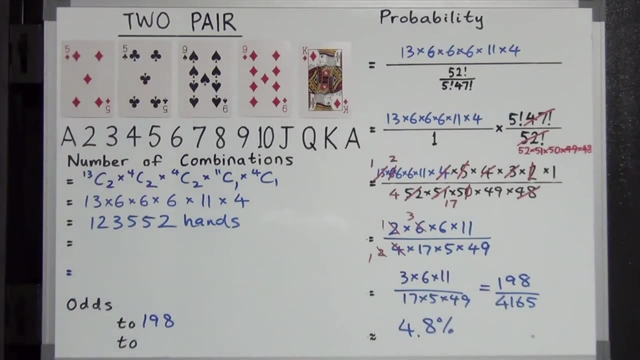 is a probability as a percentage of approximately 4.8%. So if we want to look at the odds of that, for every 4165 hands we are going to get 298, two pairs on average, And doing the subtraction there, that will give us 3,967.. 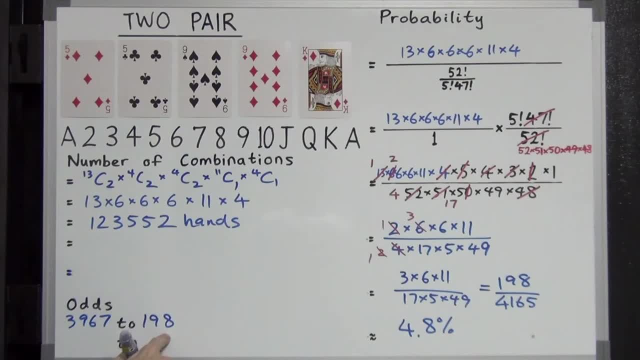 Okay, so for every 198 two pair hands you are going to get, on average you are going to get 3,967 hands that are not two pairs. Dividing both sides of this by 198, we get 1 and 20..